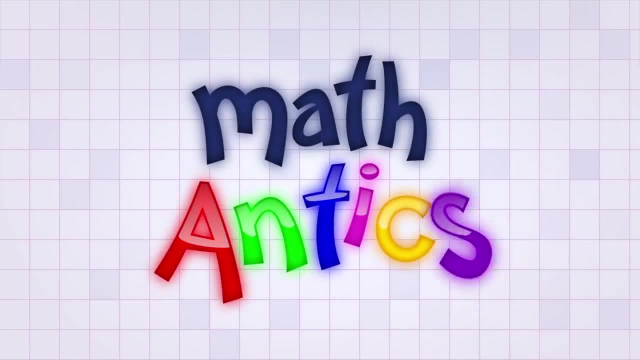 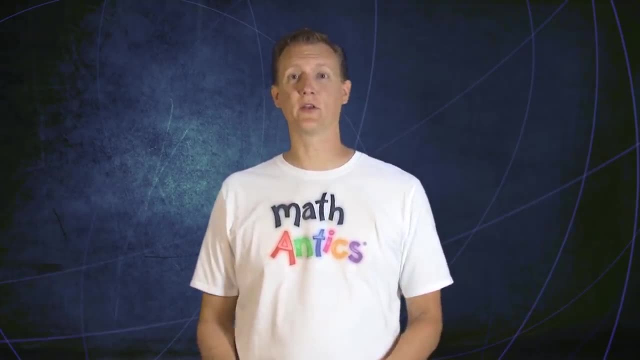 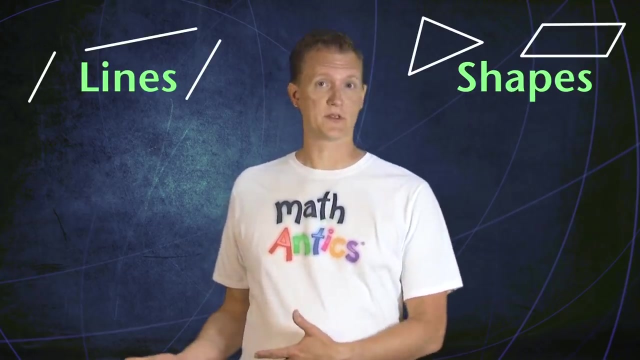 Hi there, Today, on Math Antics, we're starting a new subject where we're going to learn the basics of a special kind of math called Geometry. Geometry is the study of things like lines, shapes, angles, distances and things like that. 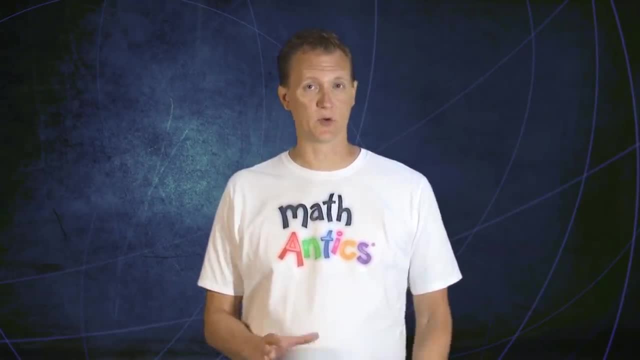 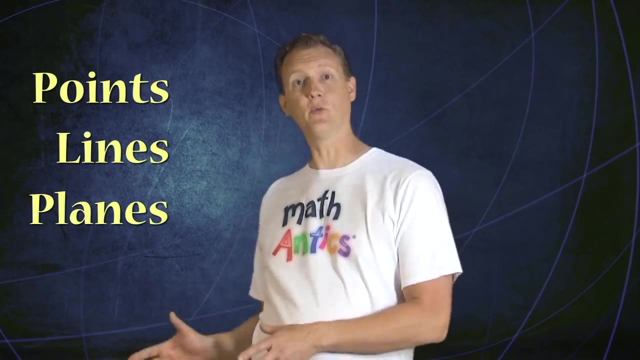 In this video, we're going to focus on three of the most basic elements or parts of geometry. They are Points, Lines and Planes. Alright, we're going to start with points, because they're about the simplest thing you can imagine in geometry. 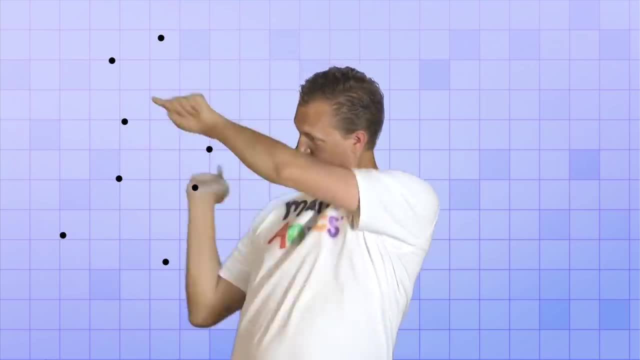 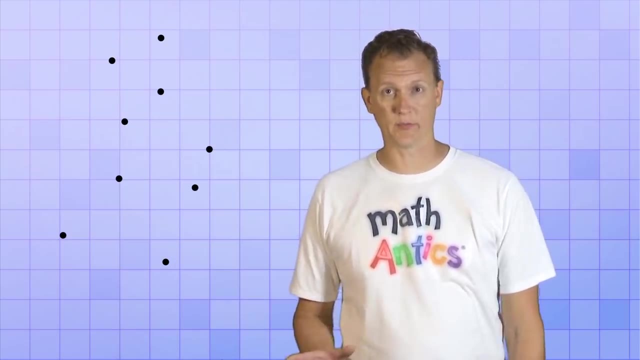 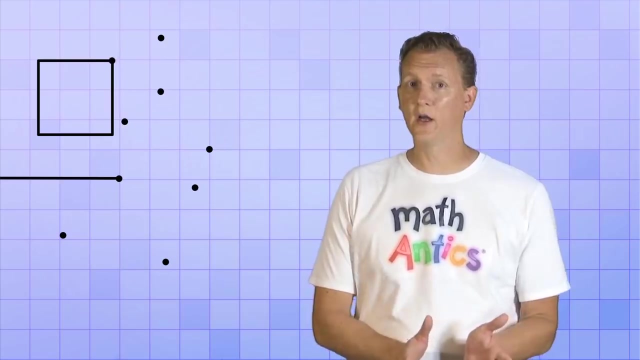 What's a point? Well, let me draw some for you. So these are points. They're just little, tiny dots in space, but they do a really important job in geometry. They help us describe specific locations in space, like the end of a line or the corner of a square. 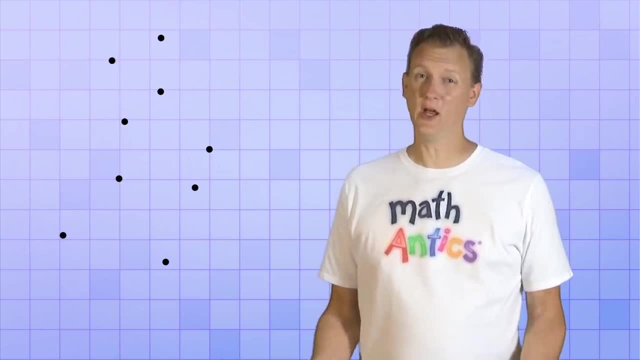 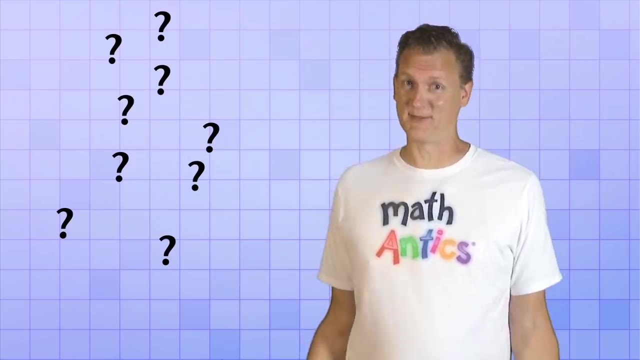 or the center of a circle, But they won't really help that much, Unless we name them, Because if I say, Hey, look at that point over there, it's kind of hard to tell which one I'm talking about. I mean, they all look the same. 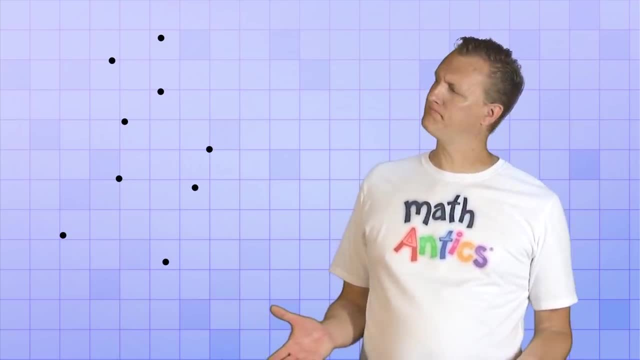 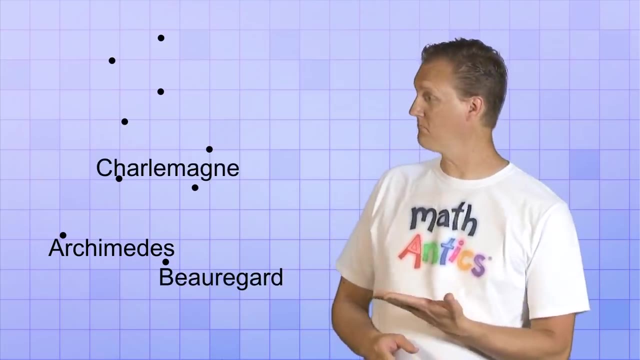 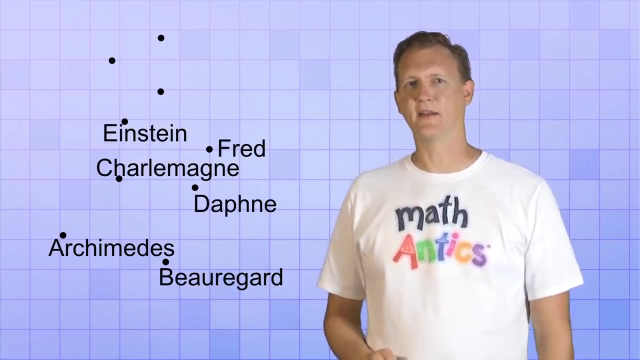 So what name should we give these points? Well, let's see, How about Archimedes and Beauregard? That'd be good. Maybe Charlemagne, How about Daphne and Einstein? Let's see Fred and Guinevere. 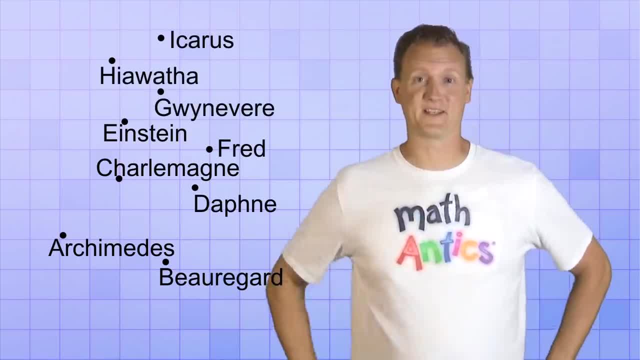 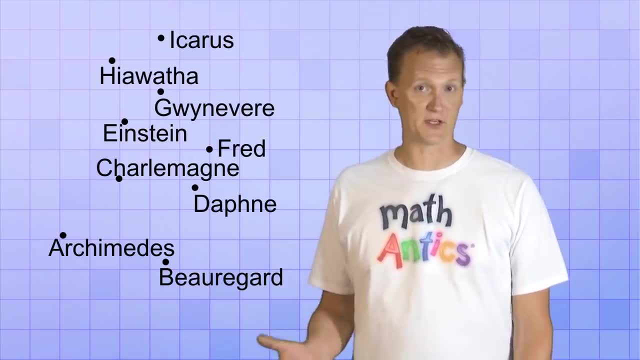 Hiawatha And Icarus- Perfect, You know. on second thought, those names are kind of long and complicated. Why don't we just use the first letters of each name instead There Now, if I say, Look at point A. 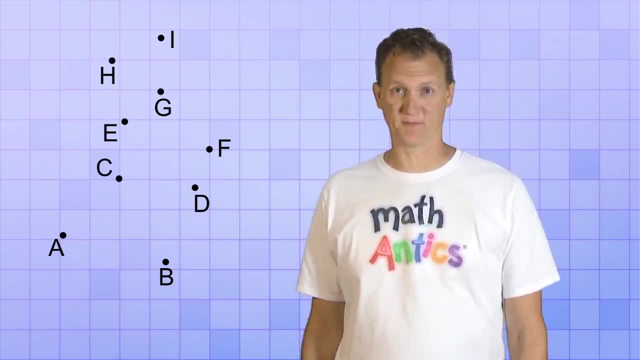 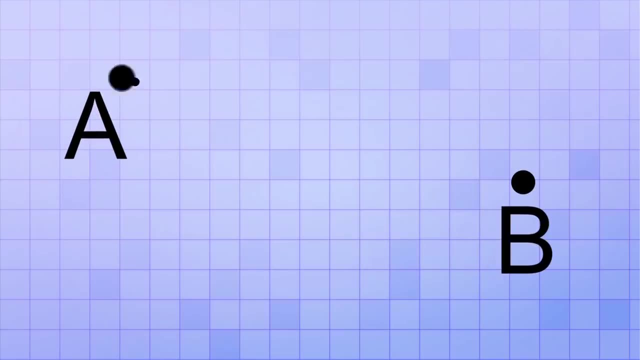 Or Look at point B. You know exactly what I'm talking about. In fact, let's do that. Let's just talk about point A and point B for a minute. If you start at point A and go to point B, taking the shortest distance possible, 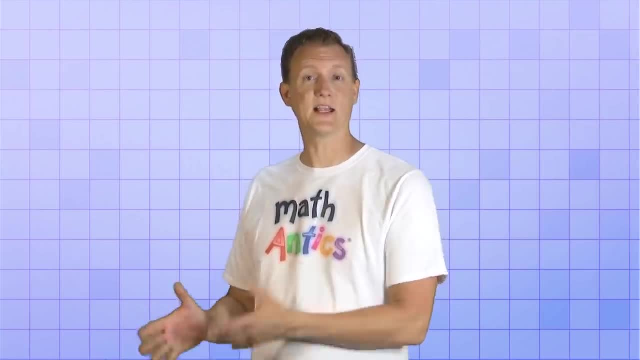 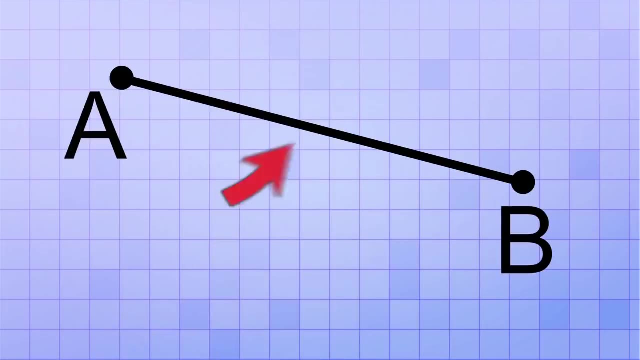 you'd have gone in a straight line. A line is the next most basic element of geometry. We name a line by the points that it goes through. For example, we would call this line AB because its end points, where it starts and stops, are points A and B. 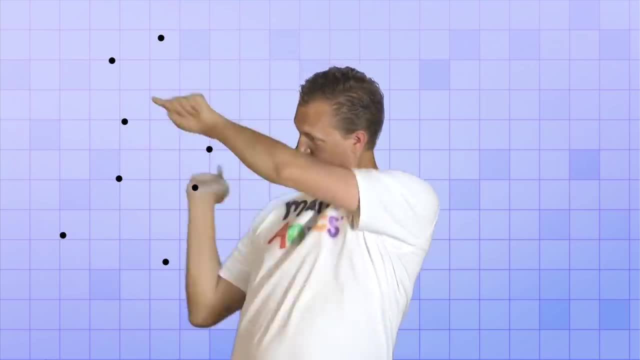 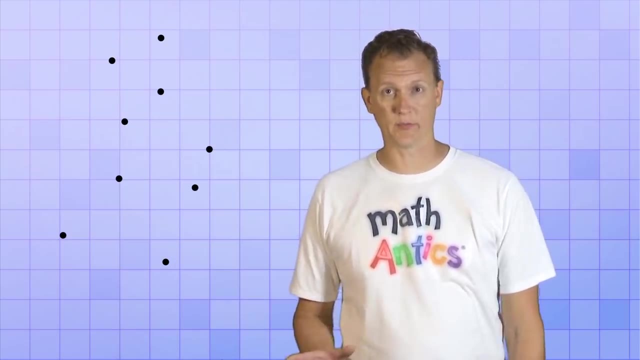 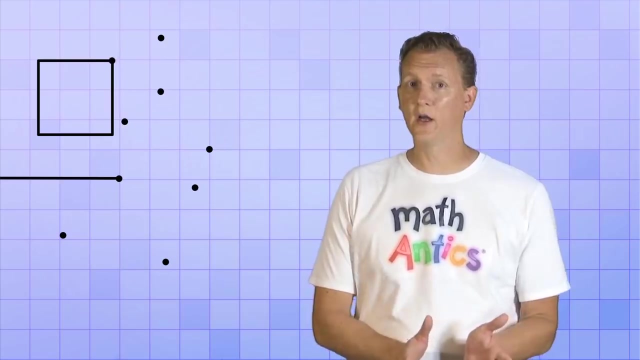 What's a point? Well, let me draw some for you. So these are points. They're just little, tiny dots in space, but they do a really important job in geometry. They help us describe specific locations in space, like the end of a line or the corner of a square. 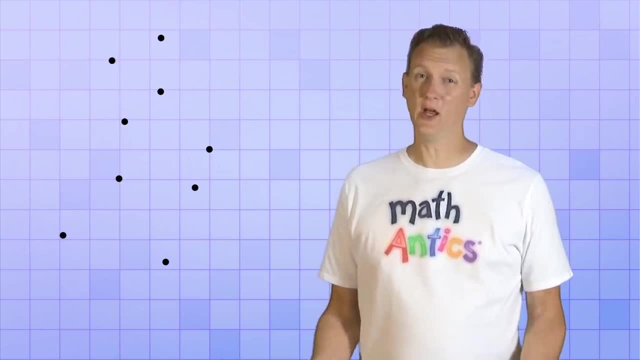 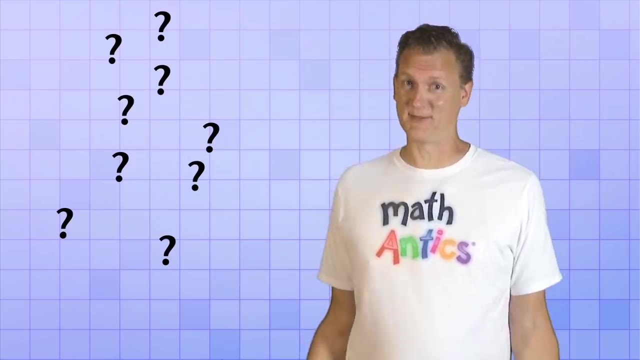 or the center of a circle, But they won't really help that much, Unless we name them, Because if I say, Hey, look at that point over there, it's kind of hard to tell which one I'm talking about. I mean, they all look the same. 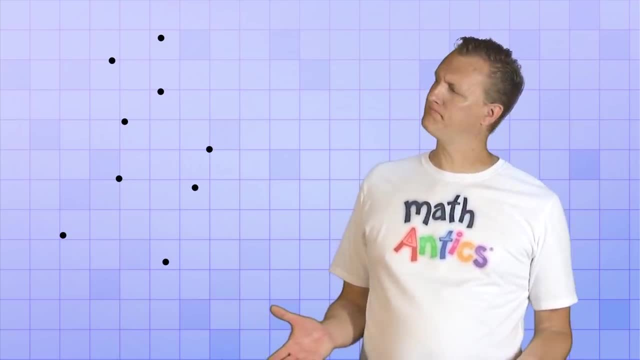 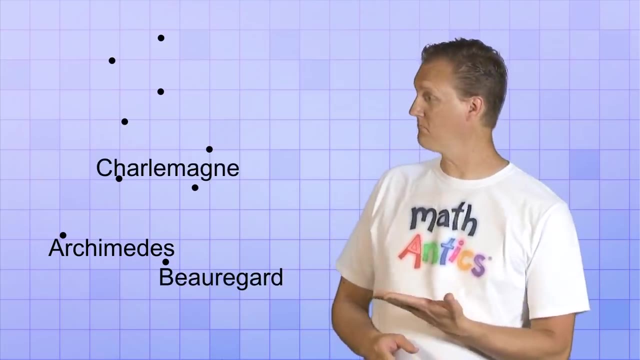 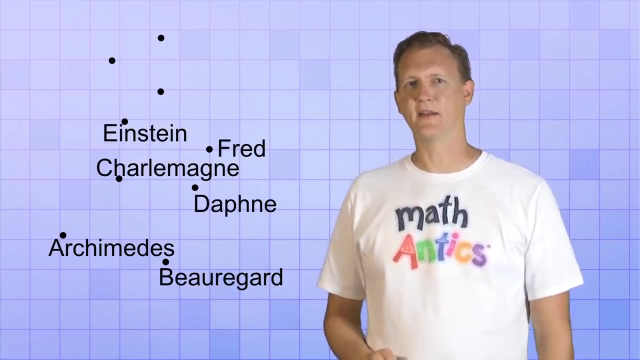 So what name should we give these points? Well, let's see, How about Archimedes and Beauregard? That'd be good. Maybe Charlemagne, How about Daphne and Einstein? Let's see Fred and Guinevere. 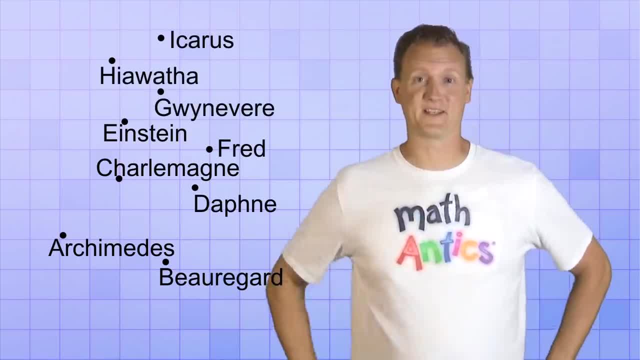 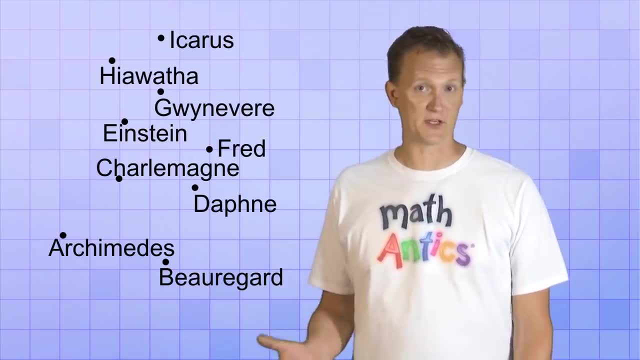 Hiawatha And Icarus- Perfect, You know. on second thought, those names are kind of long and complicated. Why don't we just use the first letters of each name instead There Now, if I say, Look at point A. 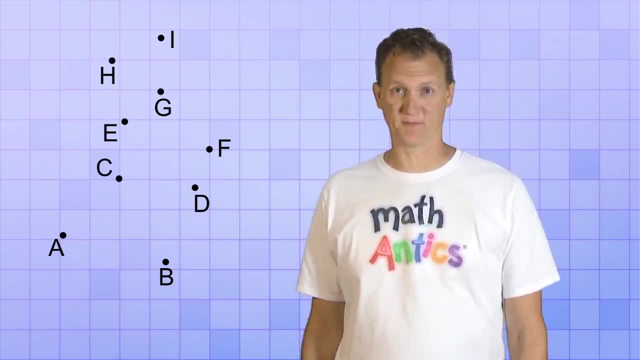 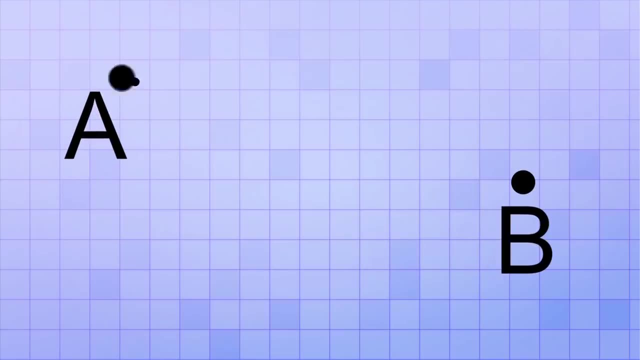 Or Look at point B. You know exactly what I'm talking about. In fact, let's do that. Let's just talk about point A and point B for a minute. If you start at point A and go to point B, taking the shortest distance possible, 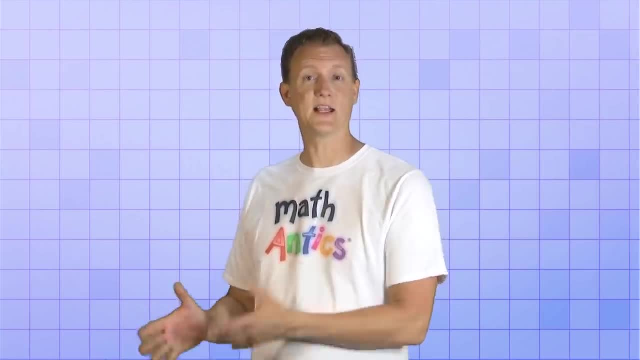 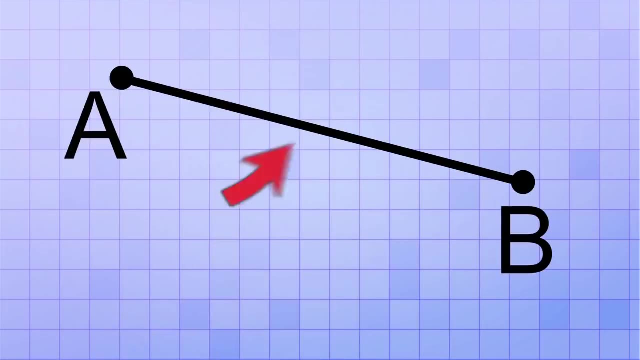 you'd have gone in a straight line. A line is the next most basic element of geometry. We name a line by the points that it goes through. For example, we would call this line AB because its end points, where it starts and stops, are points A and B. 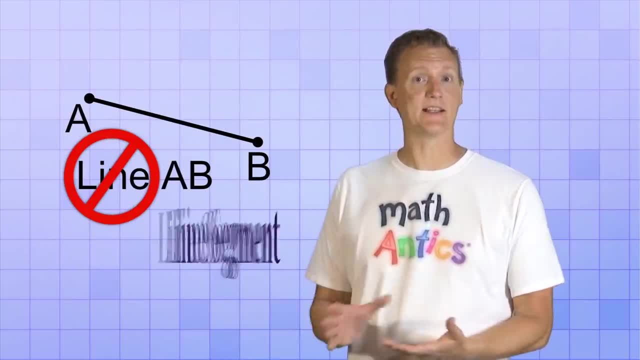 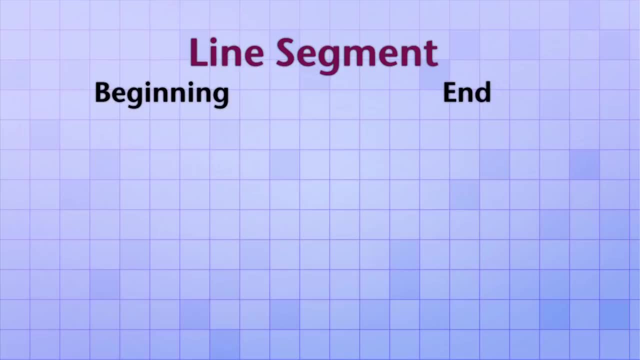 But technically this isn't really a line, It's a line segment. What's the difference, you ask? That's a good question. A line segment has a beginning and an end. It starts at one point in space and it ends at another. 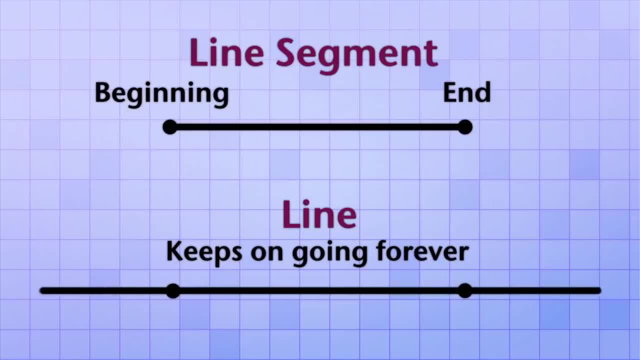 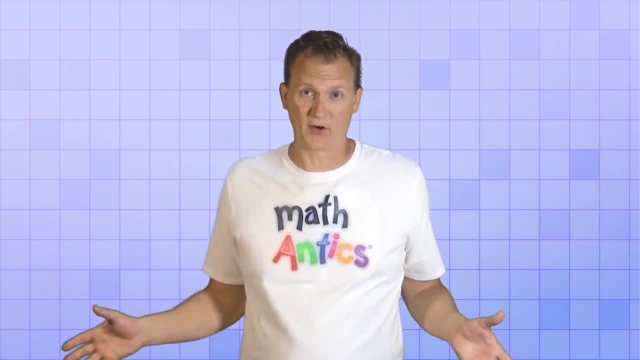 A line, on the other hand, just keeps on going in either direction forever, Just like the number line keeps on going forever. Well, at least we imagine that it goes on forever. We can't actually draw a line that goes on forever. 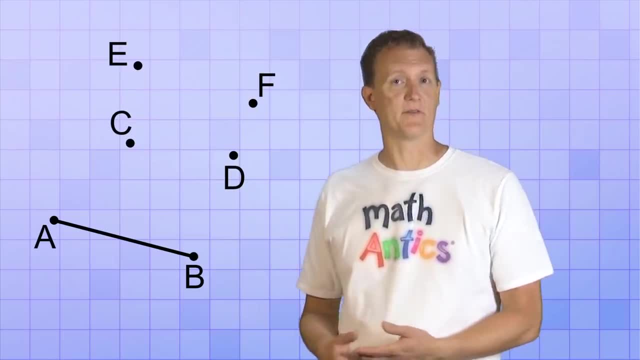 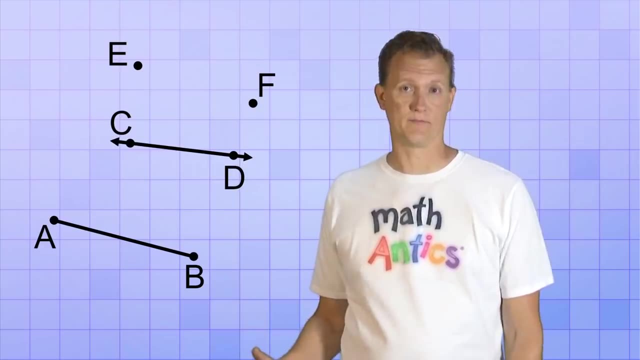 So here's what we do instead: To draw a line instead of a line segment, you just go past the end points a little bit and you put an arrow on both ends of the line to show that it keeps on going. So this is line segment AB and this is line CD. 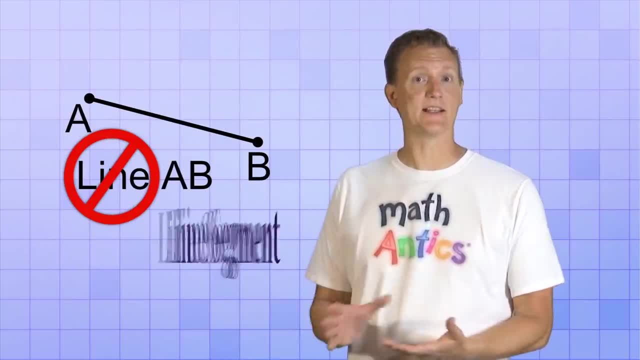 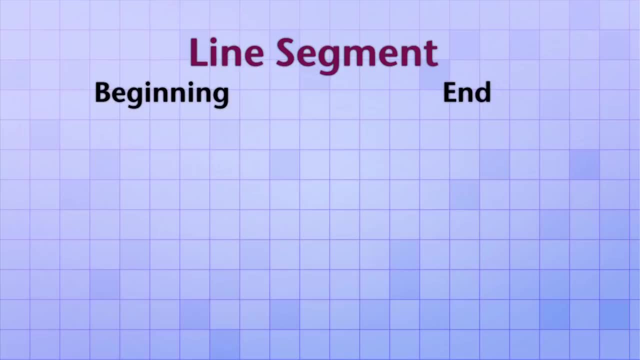 But technically this isn't really a line, It's a line segment. What's the difference, you ask? That's a good question. A line segment has a beginning and an end. It starts at one point in space and it ends at another. 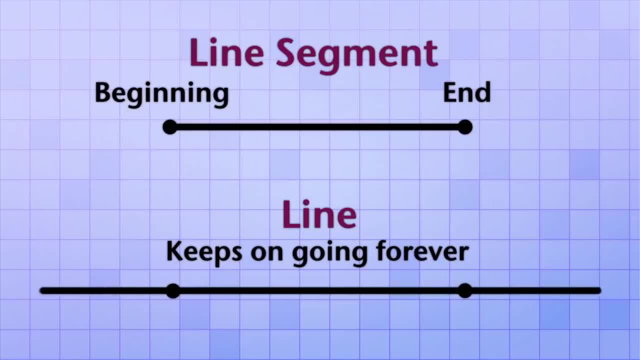 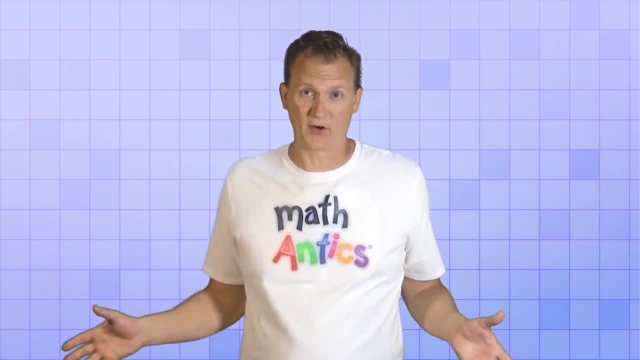 A line, on the other hand, just keeps on going in either direction forever, Just like the number line keeps on going forever. Well, at least we imagine that it goes on forever. We can't actually draw a line that goes on forever. 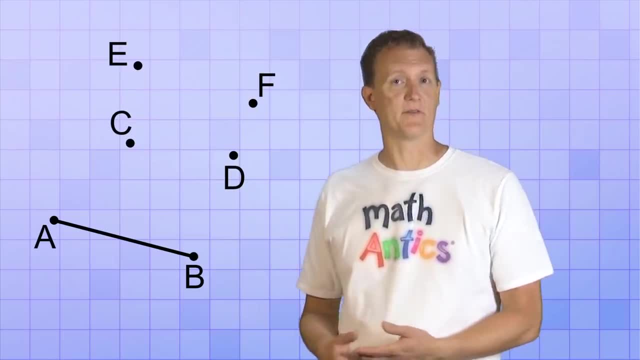 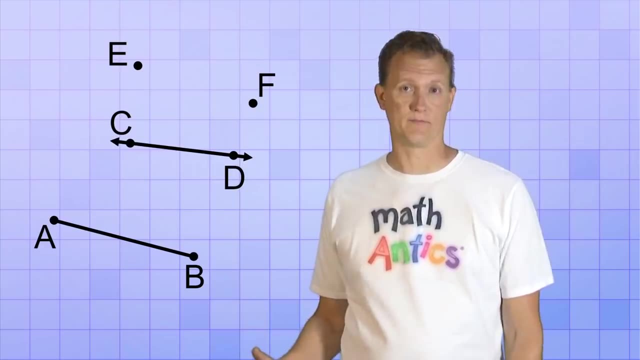 So here's what we do instead: To draw a line instead of a line segment, you just go past the end points a little bit and you put an arrow on both ends of the line to show that it keeps on going. So this is line segment AB and this is line CD. 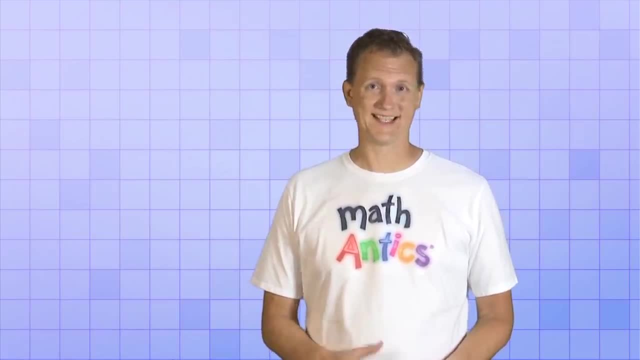 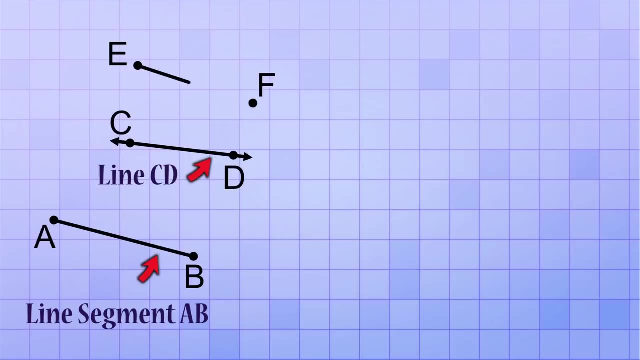 Now there's one more special type of line that we need to talk about, And it's basically a combination of a line segment and a line. We call it a ray. Rays have beginning points but no ending points. They just keep on going forever, but only in one direction. 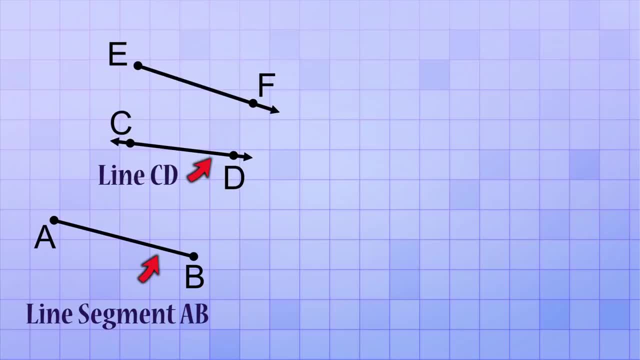 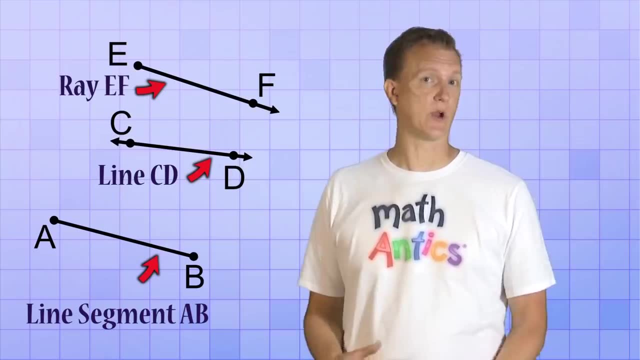 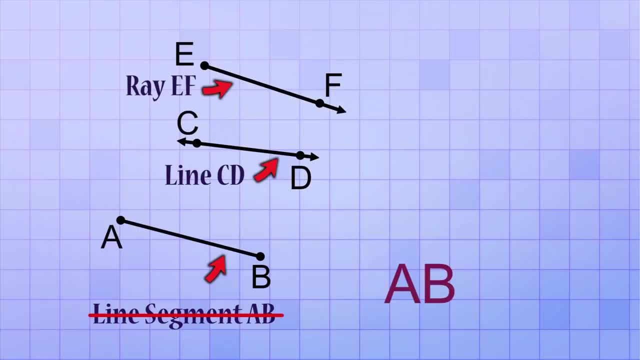 Instead of writing line segment AB, you can just write AB with a line over the top. And instead of writing line CD, you can write CD with a double arrow line over them, like this. And finally, instead of writing ray EF, you can just write EF with a single arrow line over them, like so: 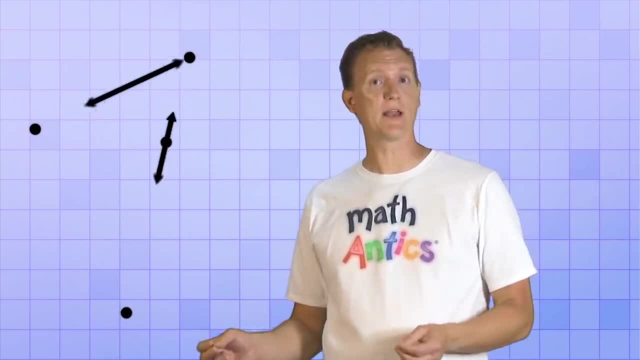 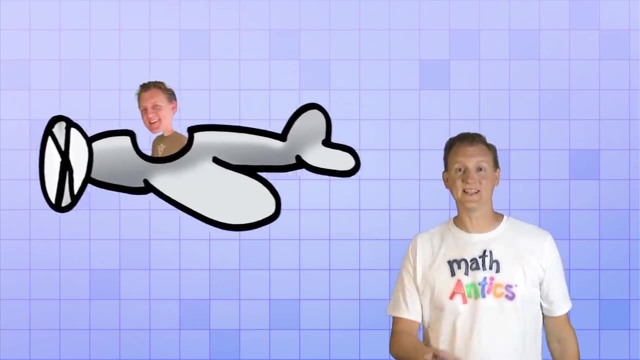 Okay, so now you know about points And you know that you can form a line between any two points. The next thing we're going to learn about is planes- No, not the kind of planes that you fly in Now, to help you understand how planes and geometry work. 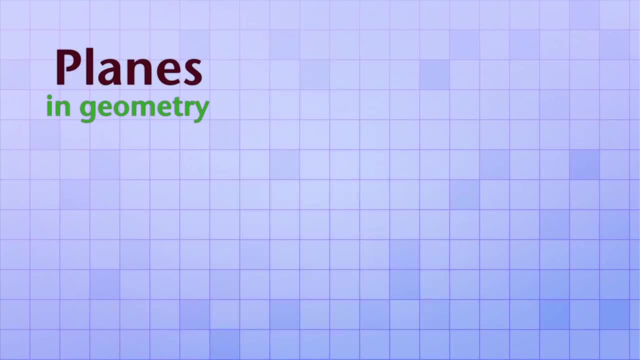 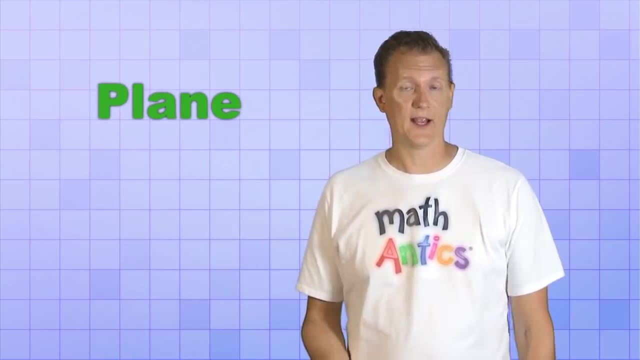 let's go back and look at all those points that we had at the beginning of the video. It looks like all the points are the same depth on your computer screen, right? And if they were, we'd say that they're all in the same plane. 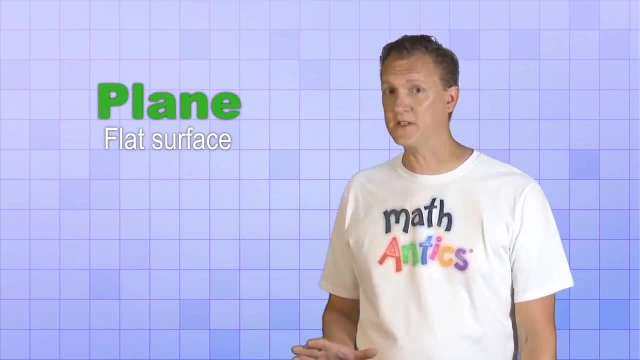 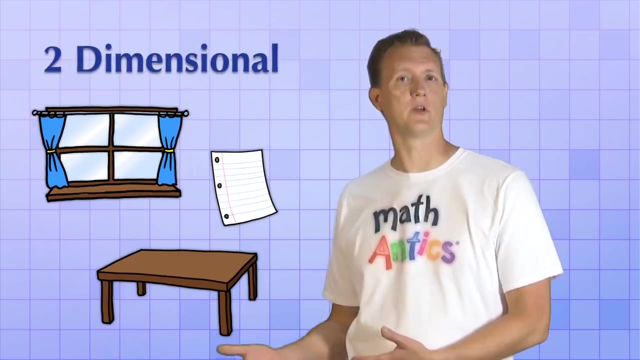 That's because your computer screen is a plane. It's a flat surface like a window or a sheet of paper or a tabletop. A plane or flat surface is what we call a two-dimensional object, because there's two dimensions that you can move in. 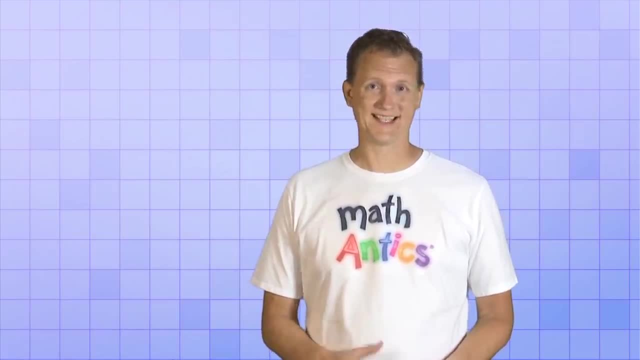 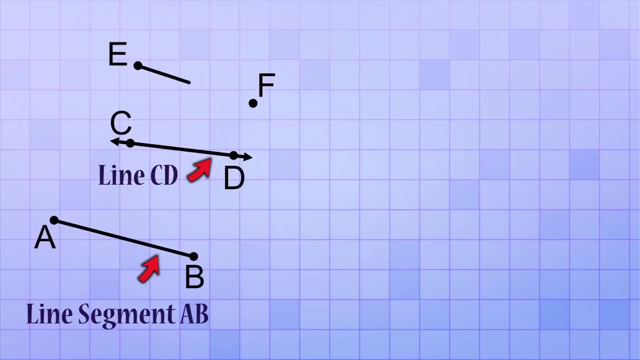 Now there's one more special type of line that we need to talk about, And it's basically a combination of a line segment and a line. We call it a ray. Rays have beginning points but no ending points. They just keep on going forever. 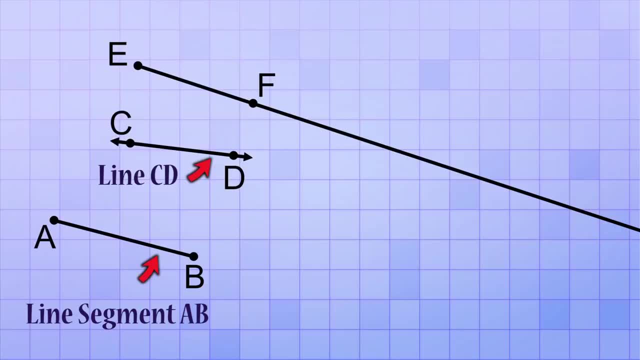 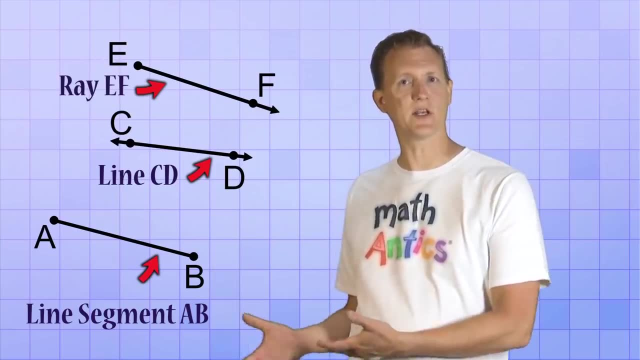 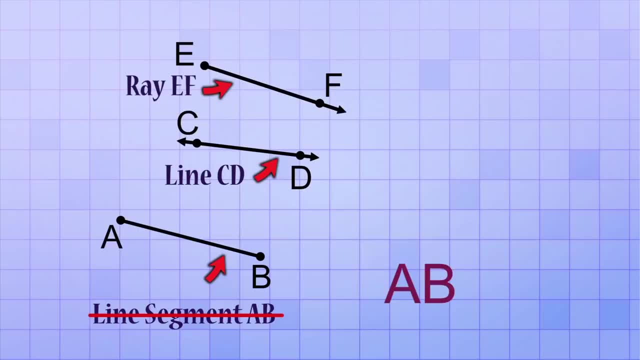 Instead of writing line segment AB, you can just write AB with a line over the top. And instead of writing line CD, you can write CD with a double arrow line over them, Like this: And finally, instead of writing ray EF, you can just write EF with a single arrow line over them. 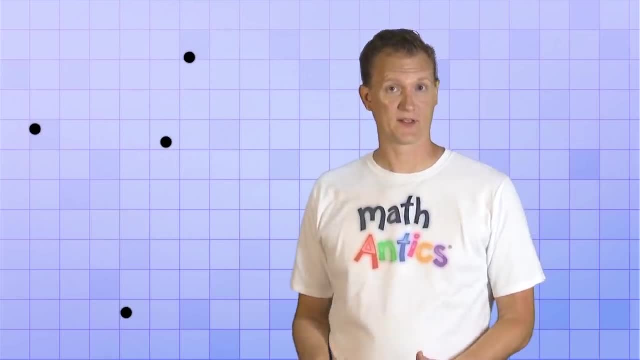 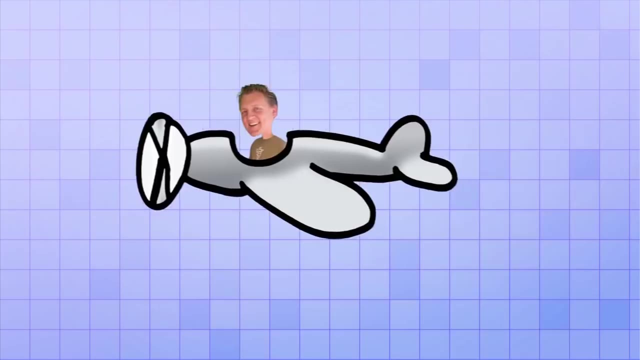 Like so. Okay, so now you know about points And you know that you can form a line between any two points. The next thing we're going to learn about is planes- No, not the kind of planes that you fly in Now, to help you understand how planes and geometry work. 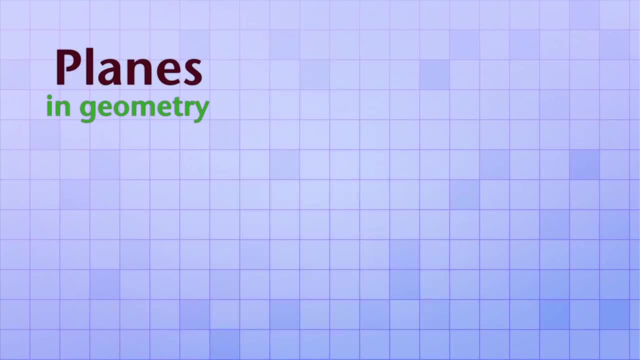 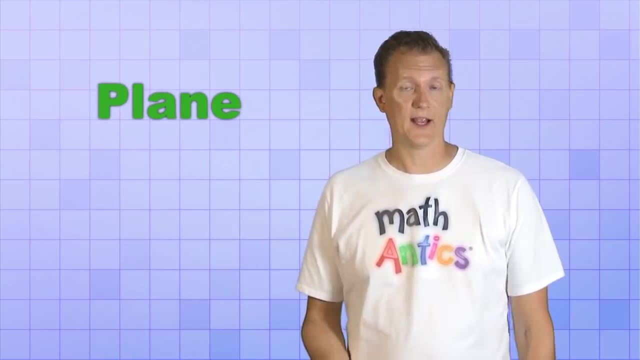 let's go back and look at all those points that we had at the beginning of the video. It looks like all the points are the same depth on your computer screen, right? And if they were, we'd say that they're all in the same plane. 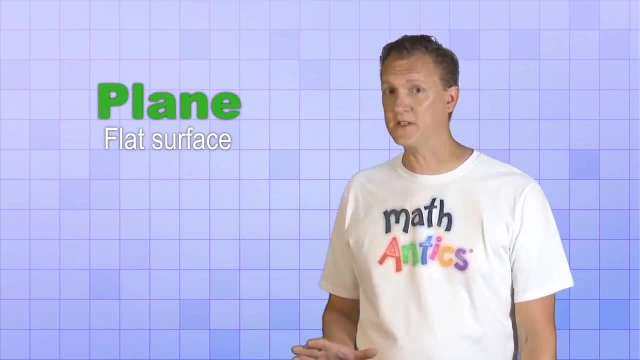 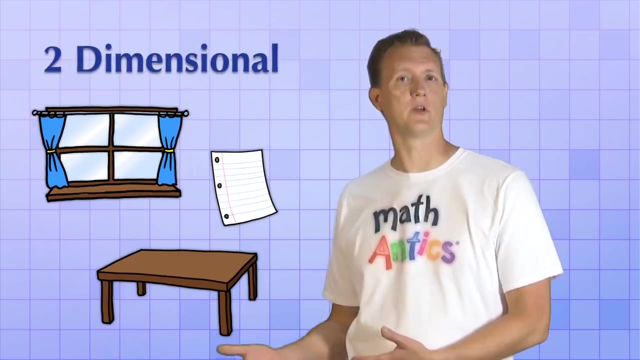 That's because your computer screen is a plane. It's a flat surface like a window or a sheet of paper or a tabletop. A plane or flat surface is what we call a two-dimensional object, because there's two dimensions that you can move in. 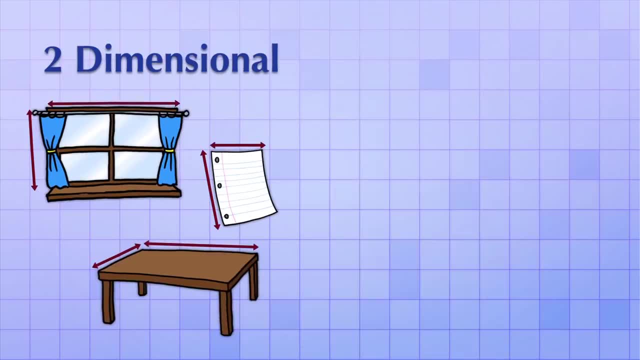 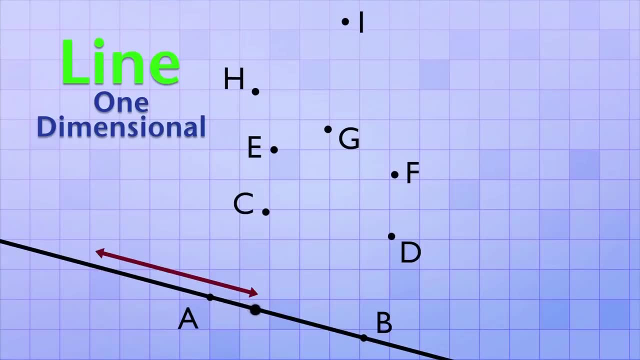 You can go up and down or you can go left and right. A line, on the other hand, is a one-dimensional object. If you're on a line like line AB, there's only one dimension that you can travel in. 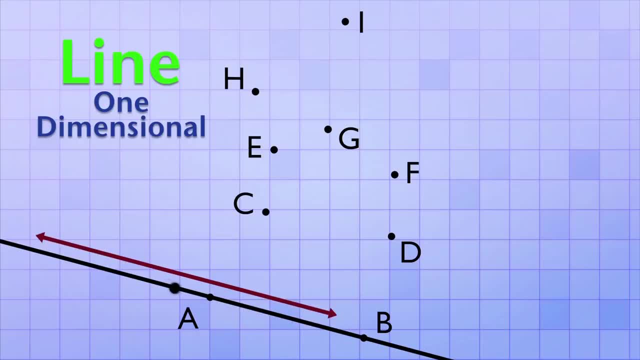 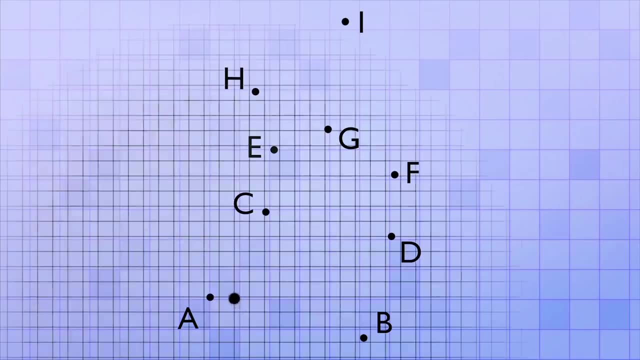 Sure, you can go forwards or backwards along that line, but it still has only one dimension. You can't get to point C without going off of line AB. But if you're on a plane, a two-dimensional object, then you can get to point C. 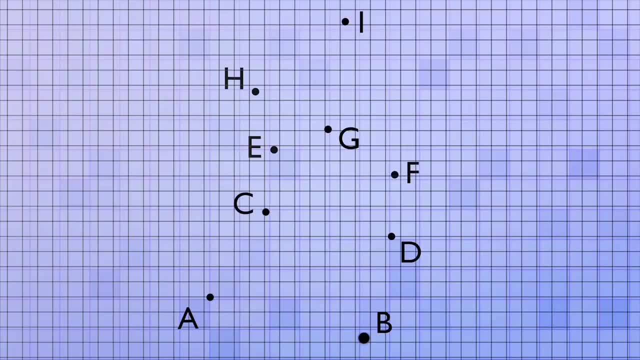 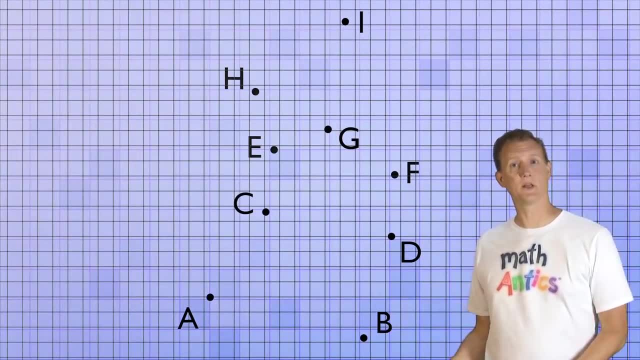 because point C is on the same plane as points A and B. Point A and point B are on that flat two-dimensional surface which is your computer screen, Cool. So that means that if I want to get to point D, I can do that too. 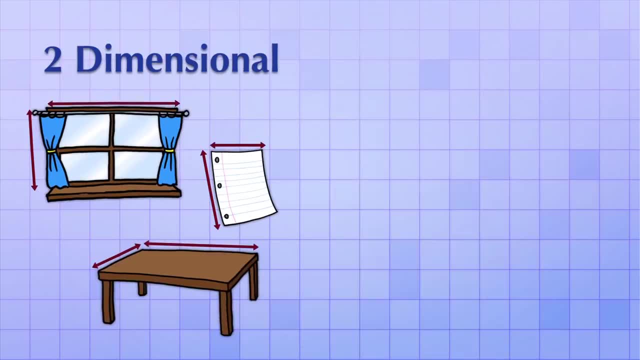 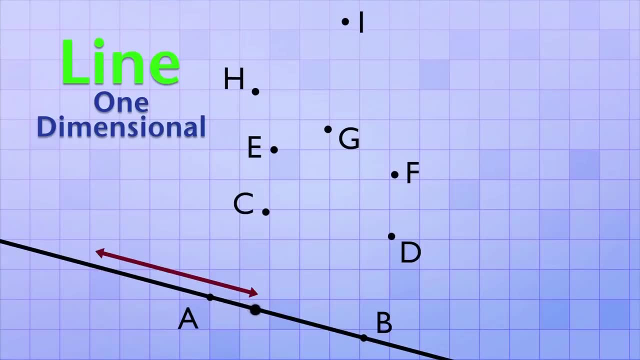 You can go up and down or you can go left and right. A line, on the other hand, is a one-dimensional object. If you're on a line like line AB, there's only one dimension that you can travel in. 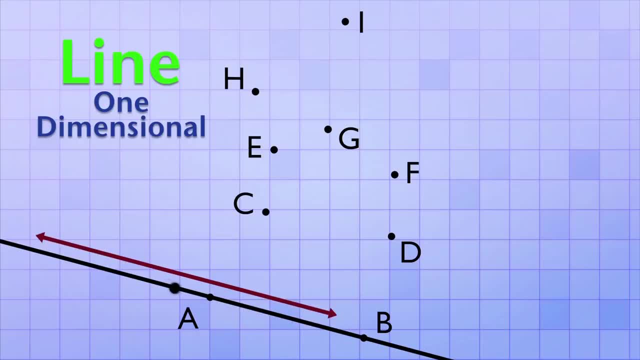 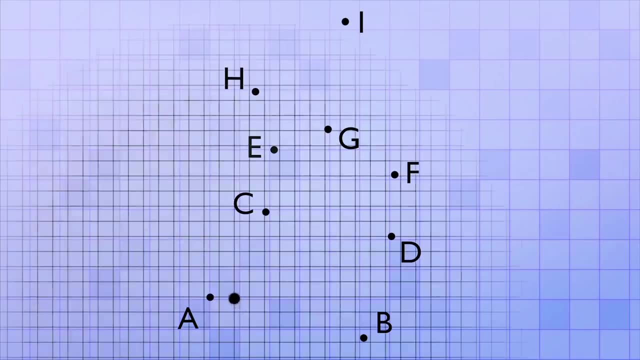 Sure, you can go forwards or backwards along that line, but it still has only one dimension. You can't get to point C without going off of line AB. But if you're on a plane, a two-dimensional object, then you can get to point C. 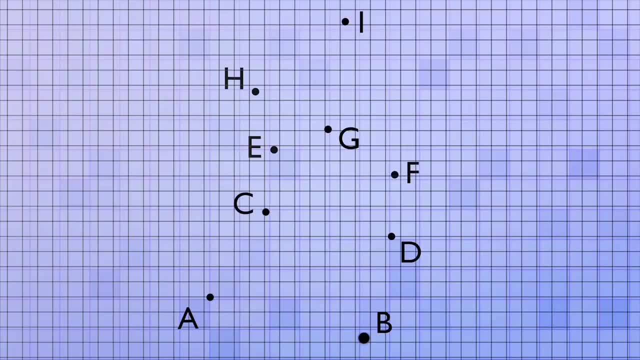 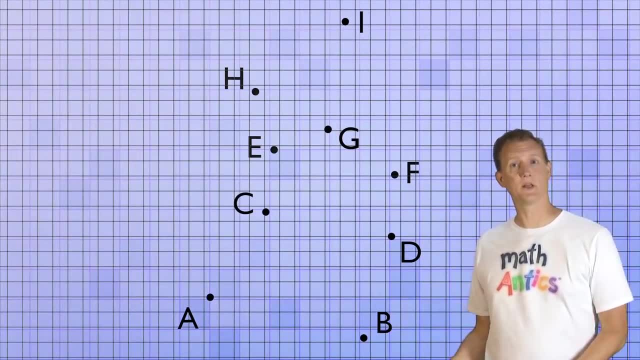 because point C is on the same plane as points A and B. Point A and C are on that flat two-dimensional surface which is your computer screen, Cool. So that means that if I want to get to point D, I can do that too. 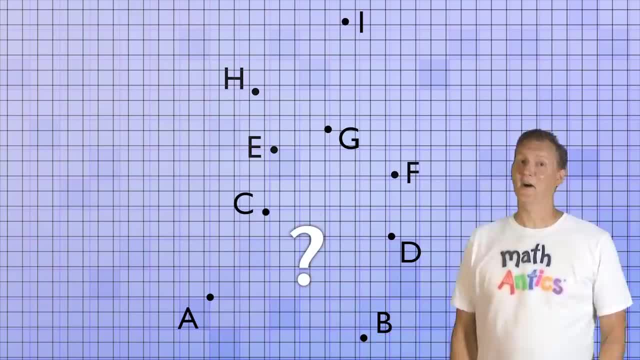 Because it's on the same plane as A, B and C. right Alright, I have a confession to make. I tricked you. Point D really isn't in the same plane as the computer screen. It just looks like it from the position you're viewing it from. 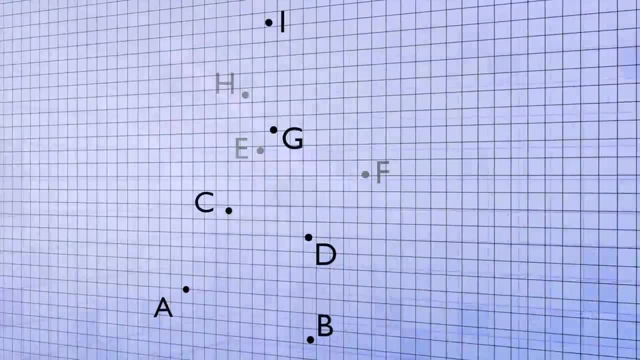 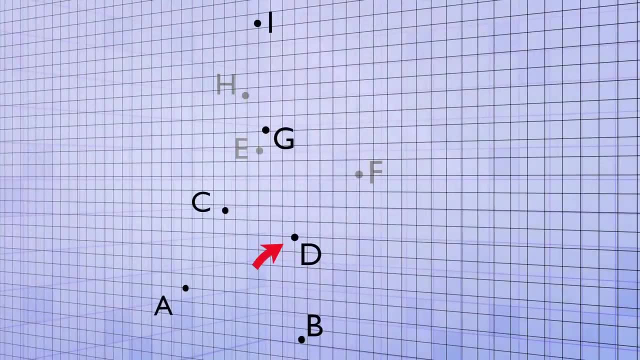 Watch what happens if I start rotating the screen. space a little bit. Aha, Now you can see that the points are actually scattered all over. the point Point D is actually in front of the plane that A, B and C were in. 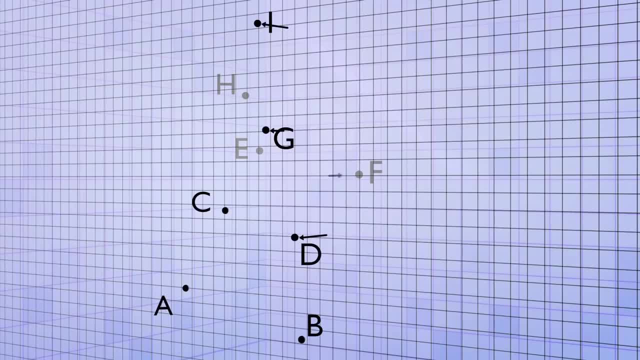 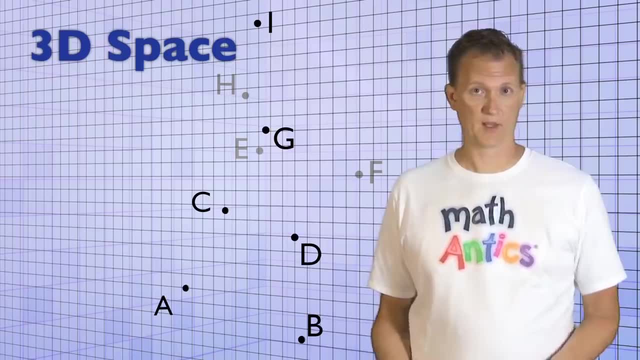 along with some of the other points, And the rest of the points are actually behind the plane that A, B and C are in. What we have here is a three-dimensional space, or 3D space for short. In a three-dimensional space, there's three dimensions you can move in. 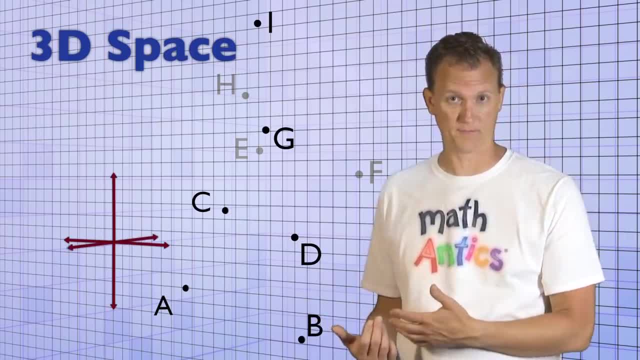 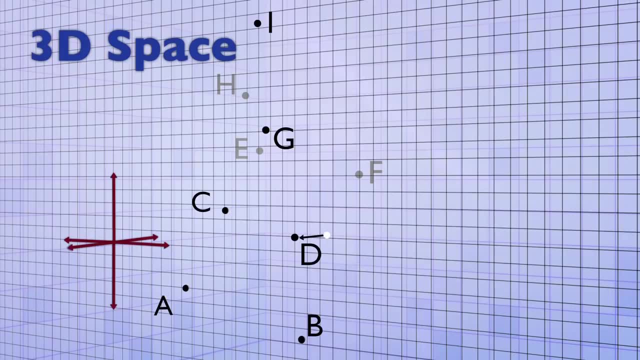 Left to right, up and down and in and out. If we're on the plane that contains points A, B and C, we can't get to point D unless we leave that plane by traveling in that third dimension, A three-dimensional space, like this is often called a volume. 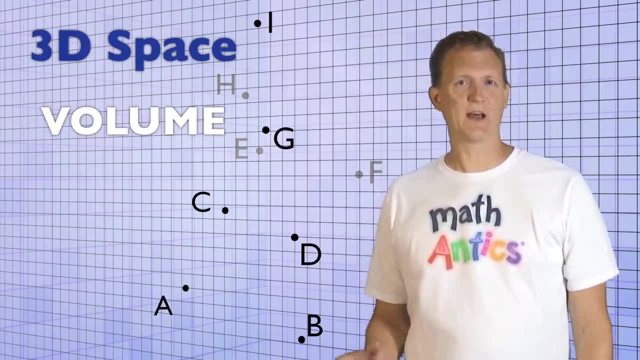 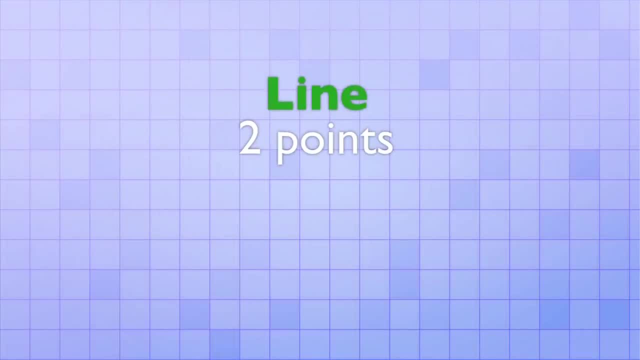 but we'll talk all about 3D volumes in another video. For now, let's get back to talking about planes. Earlier in the video, we learned that you can make a line by connecting any two points, right? Well, in order to make a plane, it turns out that you need to have three points. 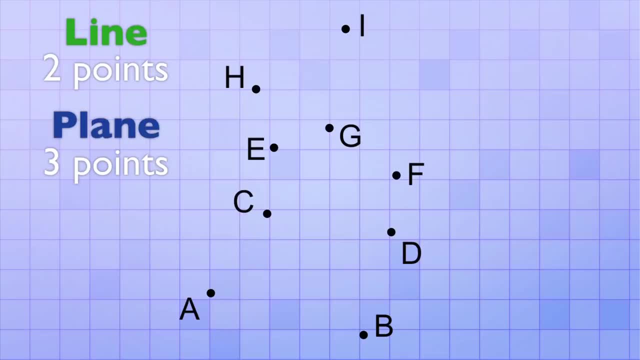 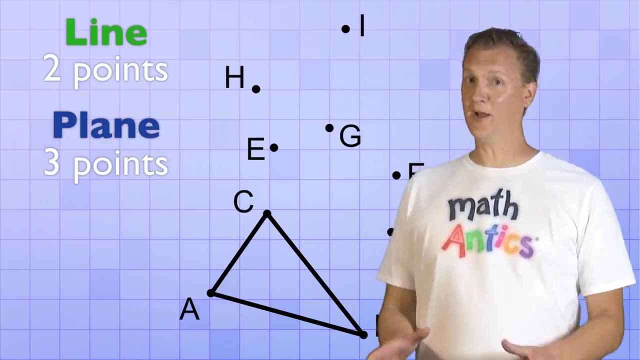 Like our three points: A, B and C. If you just connect A and B, you get a line. But if you connect A, B and C, you get a… a triangle. Now you're probably thinking: wait, I thought we were supposed to get a plane, not a triangle. 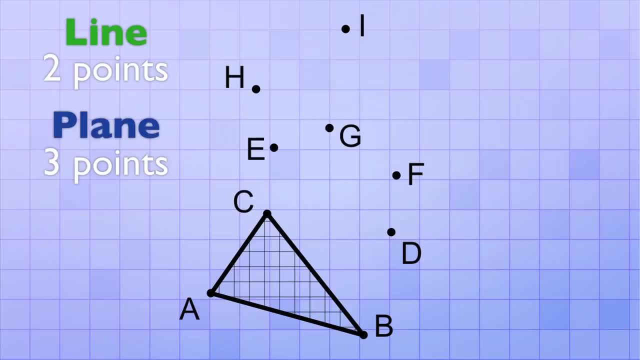 Well, because it is a flat surface. a triangle is a lot like a plane, but it has three edges. It stops and doesn't keep on going forever. When we were talking about lines, do you remember how a line segment had endpoints? 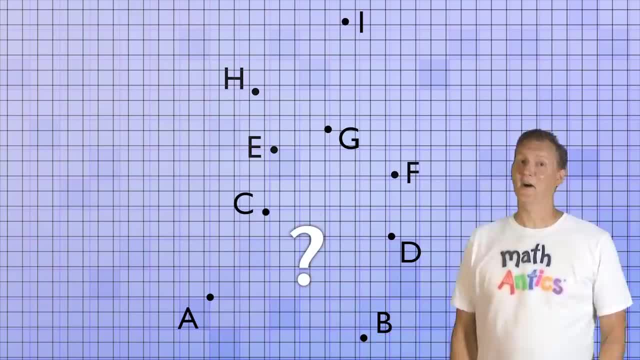 Because it's on the same plane as A, B and C, right, All right, I have a confession to make. I tricked you. Point D really isn't in the same plane as the computer screen. It just looks like it from the position you're viewing it from. 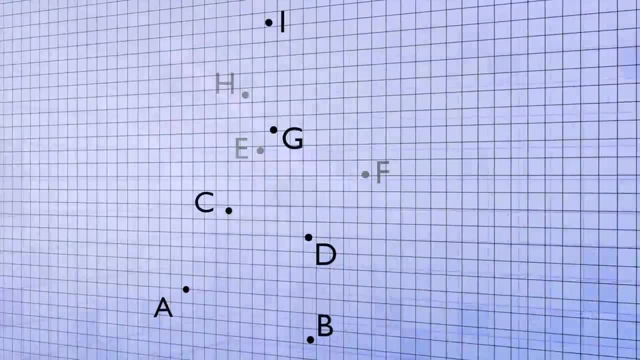 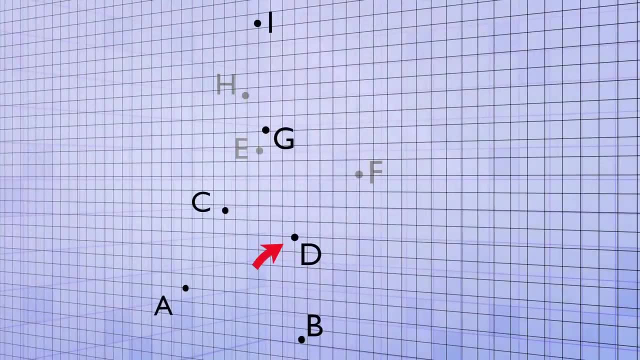 Watch what happens if I start rotating the screen. space a little bit. Aha, Now you can see that the points are actually scattered all over. the point Point D is actually in front of the plane that A, B and C were in. 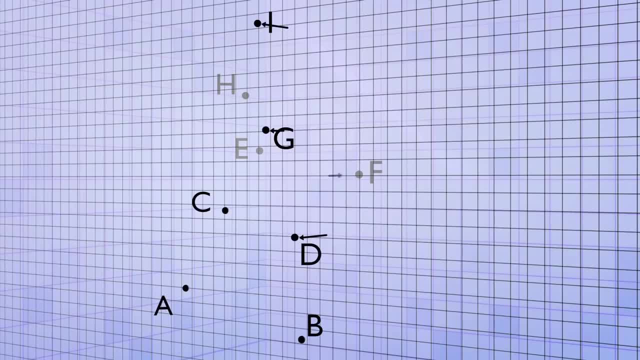 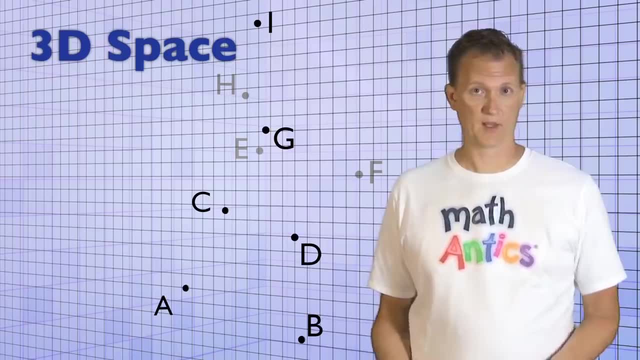 along with some of the other points, And the rest of the points are actually behind the plane that A, B and C are in. What we have here is a three-dimensional space, or 3D space for short. In a three-dimensional space, there's three dimensions you can move in. 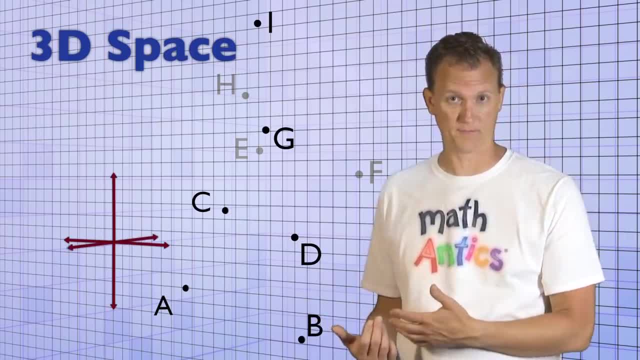 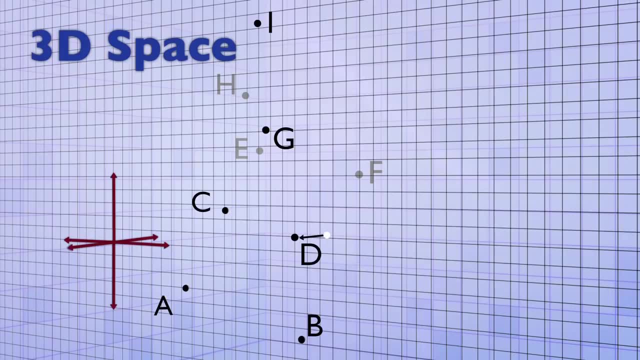 Left to right, up and down and in and out. If we're on the plane that contains points A, B and C, we can't get to point D unless we leave that plane by traveling in that third dimension, A three-dimensional space, like this is often called a volume. 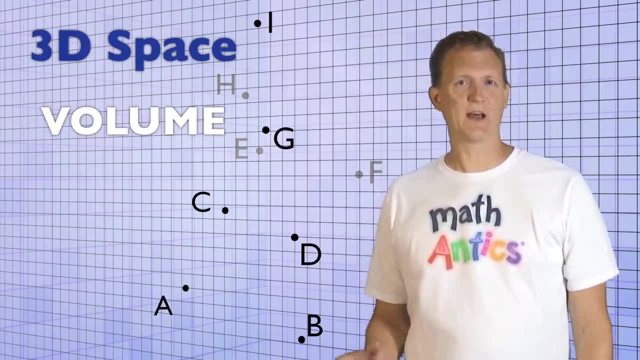 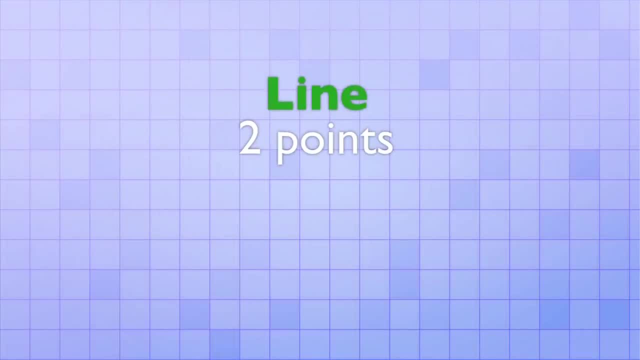 but we'll talk all about 3D volumes in another video. For now, let's get back to talking about planes. Earlier in the video, we learned that you can make a line by connecting any two points, right? Well, in order to make a plane, it turns out that you need to have three points. 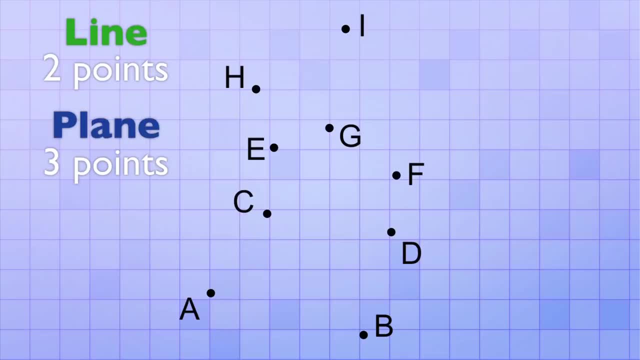 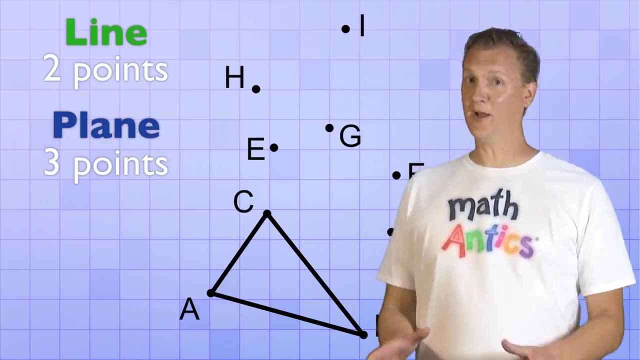 Like our three points: A, B and C. If you just connect A and B, you get a line. But if you connect A, B and C, you get a… a triangle. Now you're probably thinking: wait, I thought we were supposed to get a plane, not a triangle. 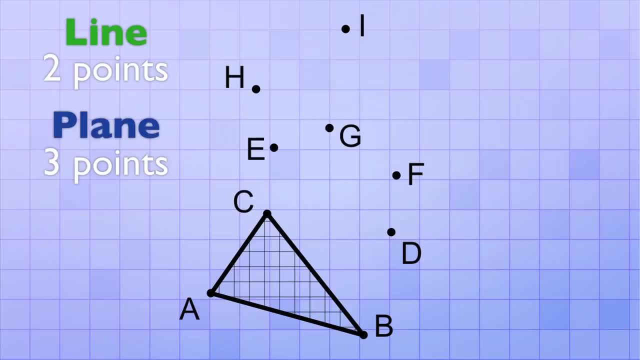 Well, because it is a flat surface. a triangle is a lot like a plane, but it has three edges. It stops and doesn't keep on going forever. When we were talking about lines, do you remember how a line segment had endpoints? 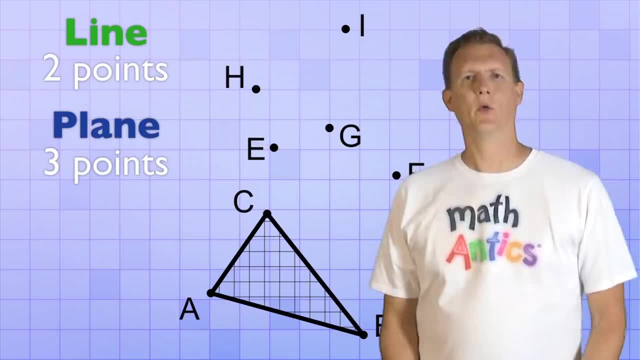 but a true line, kept on going forever. Well, it's kind of the same way with triangles and planes. You can think of a triangle as a smaller part or a segment or a segment of a plane, But the plane itself keeps on going forever. 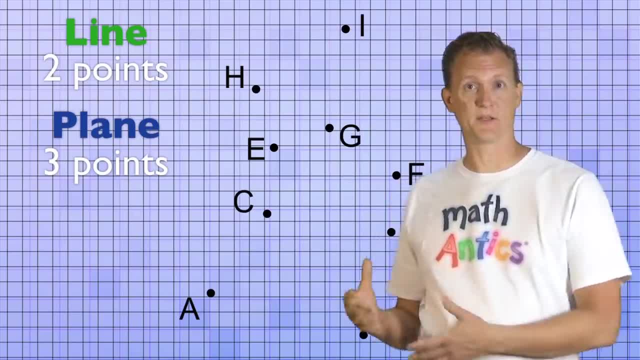 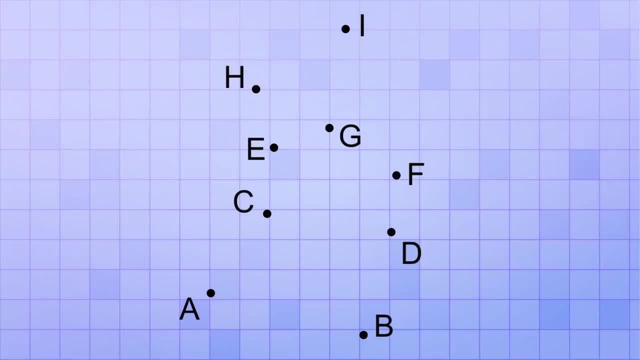 So three points is all it takes to define a plane, And in the space we've been looking at we already have plane A, B, C, So let's try making some other planes. with the rest of the points. We can choose any three points that we want to. 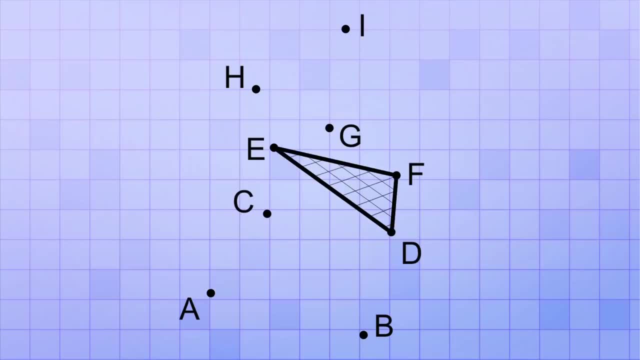 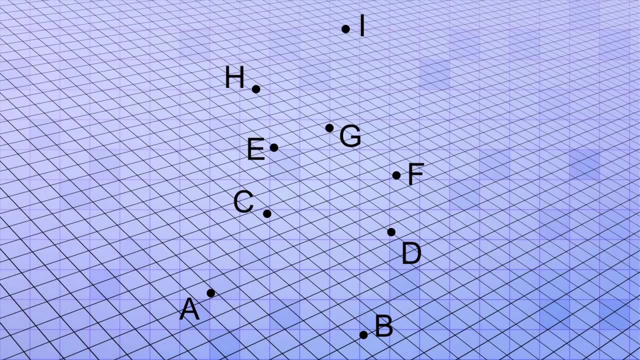 Let's join D, E and F. Now we can see the triangle they form, and if we extend that flat triangle we can see the plane that it defines. Let's try one more. so the rest of the points don't feel left out.